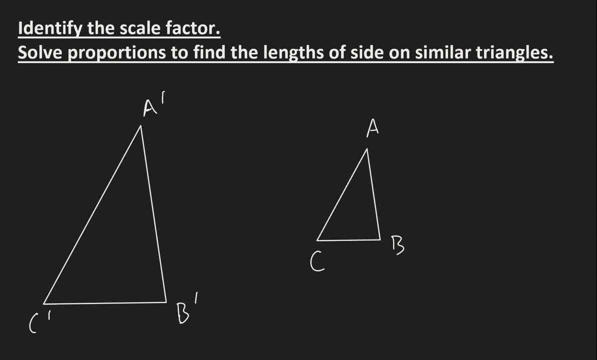 the lengths of missing sides. So if I see this triangle, I can see triangle ABC to the right and I see triangle A prime, B, prime, C prime to the left. I understand that this is scaled and actually it's increasing in size and the direction of the scaling is from the smaller ABC to the 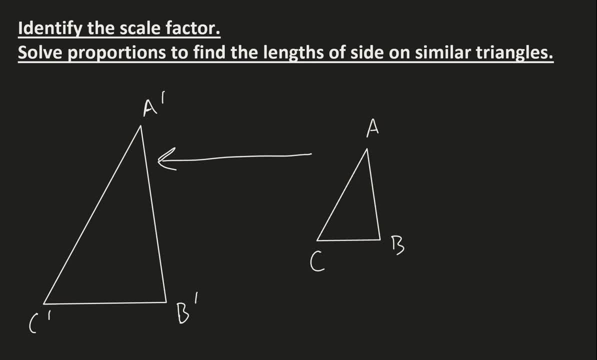 larger, And that just has to do with the fact that we know that after a transformation, we tack on the primes. So, without that arrow even being there, I understand that I'm going from the smaller one on the left to the larger one on the right. Now, having said that, I understand that my scale 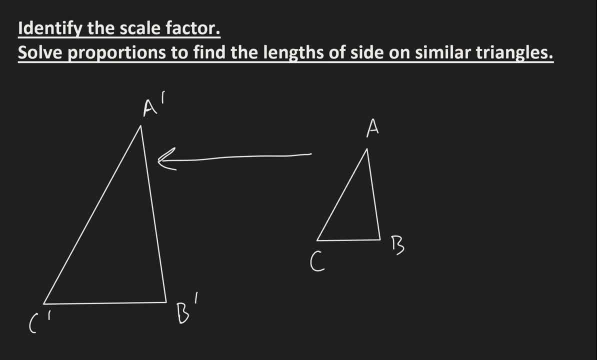 factor is going to be the same as the larger one on the right. So I'm going to go from the smaller one on the left to the larger one on the right, So my scale factor has to be a number larger than one, because I'm clearly increasing this shape. Now, if I was to say that this was three units long, 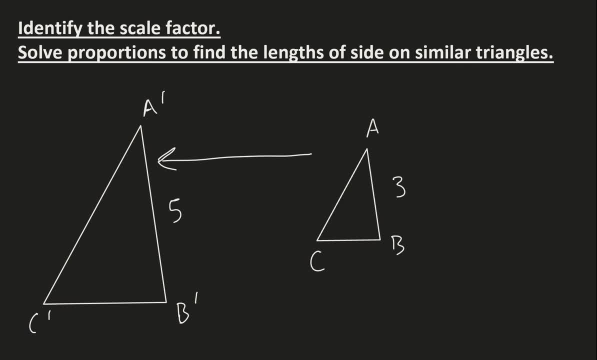 and this was five units long. my scale factor is the new or scaled up version divided by the old or the original shape. So my scale factor- you can see I land my new, my new dimension is five and the original one is three. So my scale factor is five thirds. 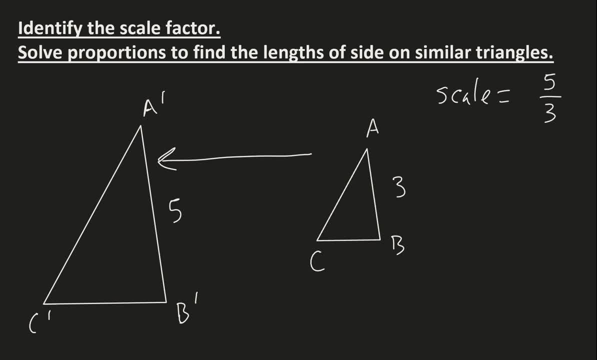 Now, if I think about that, I can take any of the dimensions of abc and if I multiply those dimensions by five thirds, I'll get the new dimension. The obvious one is the one that i have here. If I take 3 right and if i multiply that by five thirds, i should get five and, sure enough, three times. 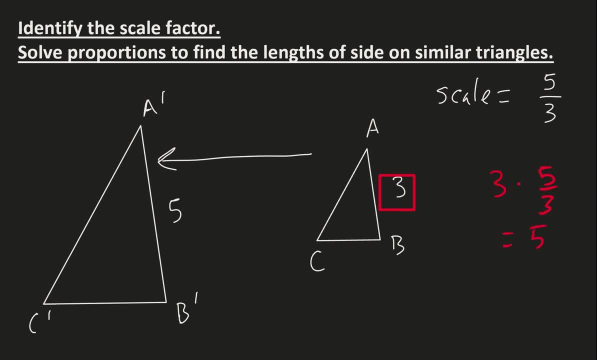 five thirds does indeed equal five. So this is the scale factor that allows me to map between the original shape and the scaled up version. let's say that i have a little bit more information on the triangle. i'll say that this dimension is uh. i'll say this is four. 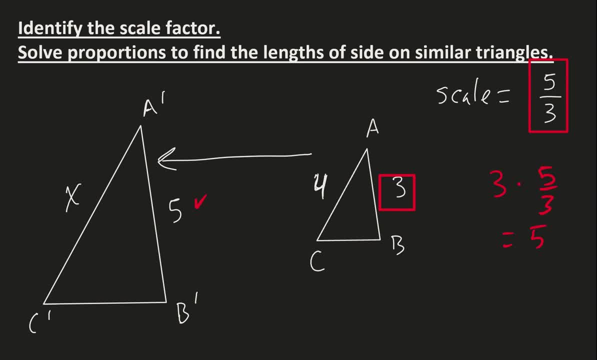 four and a question could be: what's this dimension? and maybe i'll say this is y units long and i might say that this is x units long. so now i have two additional questions. i'm asked to figure out the length of a prime, c prime which is marked with x, or i'm asked to find the length. 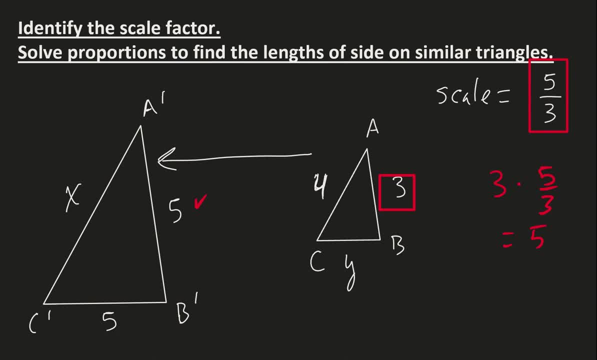 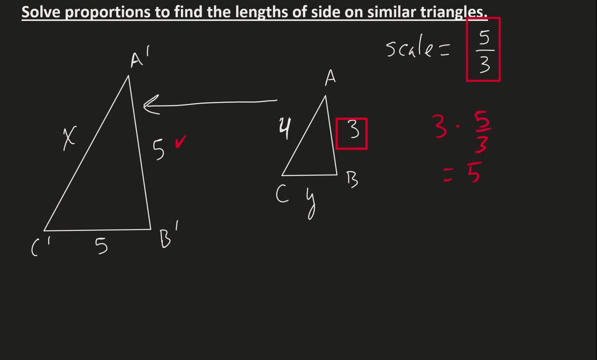 of cb, which is marked with a, y, and in both of these cases there's actually two different and similar and related methods. right, i can take the one on my original shape, for example the four, and i could multiply that by the scale factor, and that would give me x. it would give me that length. well, four times five thirds would be. 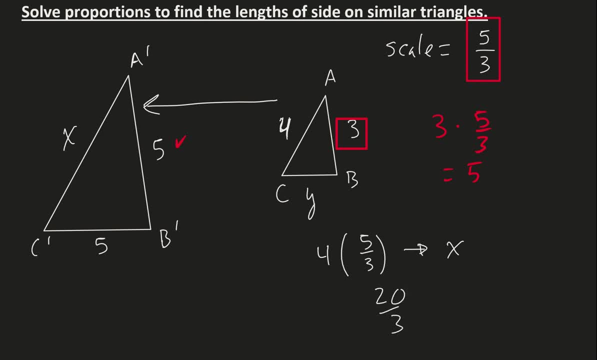 twenty thirds, and i could say that that's what x is right. x is twenty-thirds and that's a perfectly fine answer. if i wanted to, i could write it as a mixed number or i could even give it as a decimal approximation. the decimal approximation is problematic. 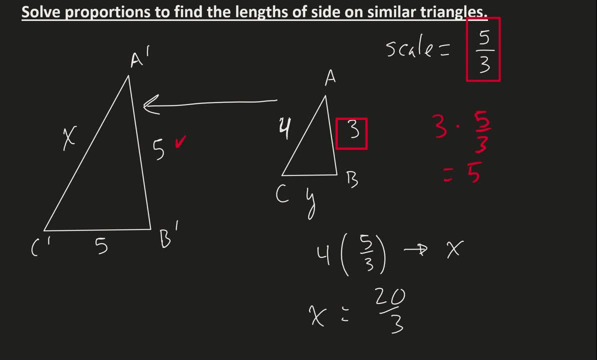 um, because it's a non-terminating decimal. that's right, it's, it's what is it? six point six, six, six, a bunch of values of six and uh, so probably twenty-thirds is the best answer. and again, um, i'm just, i'm just using this this: the fact that any dimension on my original triangle 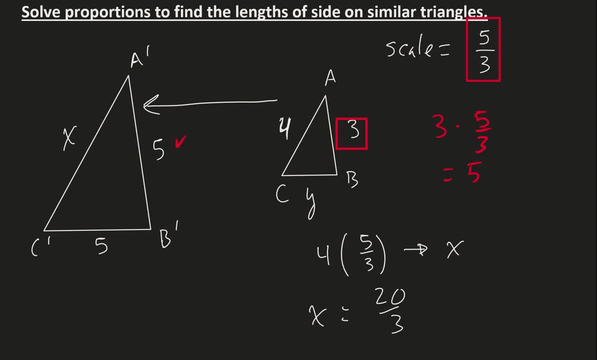 times the scale factor is going to give me the corresponding dimension on my new triangle. now i can use what i just said to figure out the length of my original triangle. and i can use what i just said to figure out the length of my original triangle. and i can use what i just said to figure 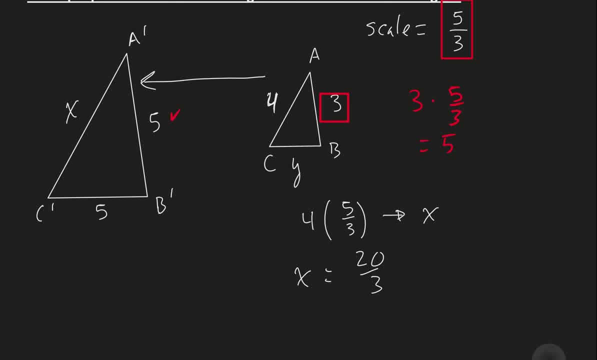 out the length of the length of y as well. however, this time y is on the original shape. so i'm going to multiply that by the scale factor. so you can see i'm going: original dimension y times my scale factor five-thirds, and that has to give me an answer of five. so now i'm just to solve. i'm 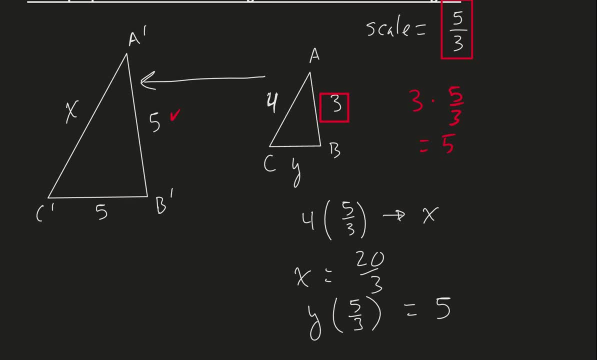 solving this equation here, to figure out what y is, what the length of y is. and i can get it one of two ways. i can divide both sides by five-thirds, or also i can notice that if i take the number five thirds and, for example, I'll just squeeze this in here and I'll write it in a 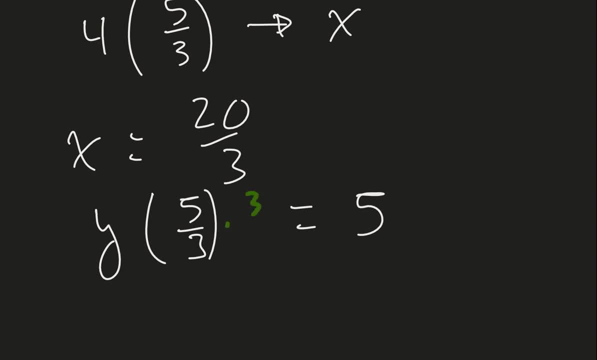 slightly different color and I multiply this side by the reciprocal of five thirds times three, fifths times three fifths. well, it turns out that five times three fifths is just the number one. so I do get Y on this side and over on the other side. I end up getting three. so why the length of this segment here would? 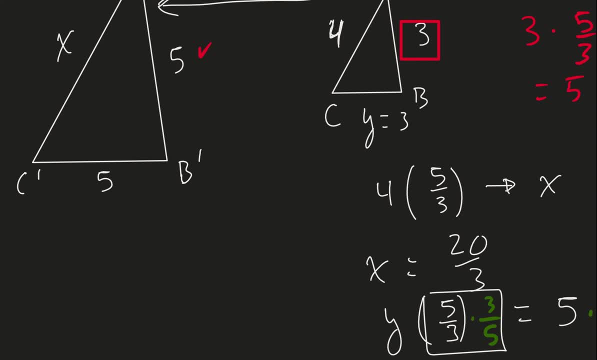 have to equal three. if this diagram was accurate- and that's kind of goofy- I should have noticed that right away, because this was already a five right, so it would follow that these would have to be the same. and what's really goofy is that this is clearly not drawn to scale, because neither one of these look like I. 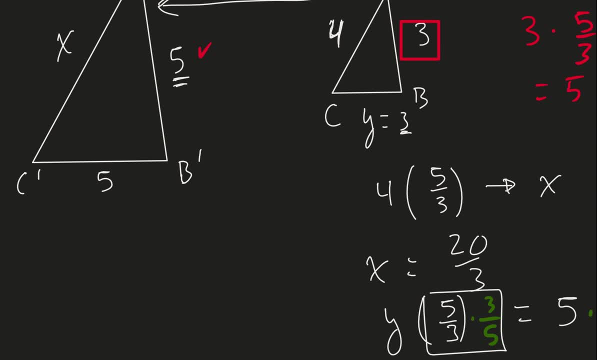 saw these triangles. there's another way that's worthy of your consideration for solving these, and I think it's something that perhaps you did in the middle school quite a bit, and that's just writing a bunch of equivalent fractions. and I think it's something that perhaps you did in the middle school quite a bit, and that's just writing a bunch of equivalent fractions. 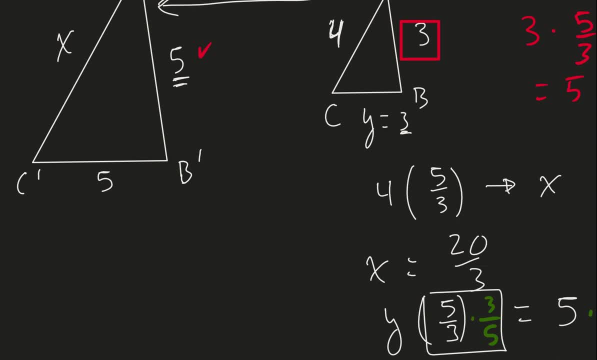 these all form proportions, so I could say, for example, I'll just go: three over five is proportionate to four over X is proportionate to Y over five, and all I'm doing is I'm just looking at this and in this case I'm taking the dimensions of 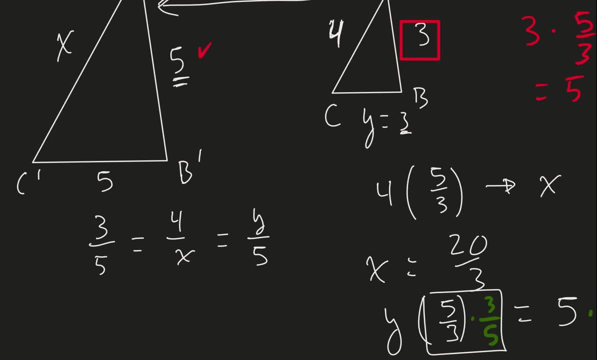 the original shape and dividing it by the new, and there's no reason why I would have to do that. I could flip these as well, and this would also be equally true. what's nice about writing it this way is that now I can actually see my scale factor at the same time. oops, I want to. 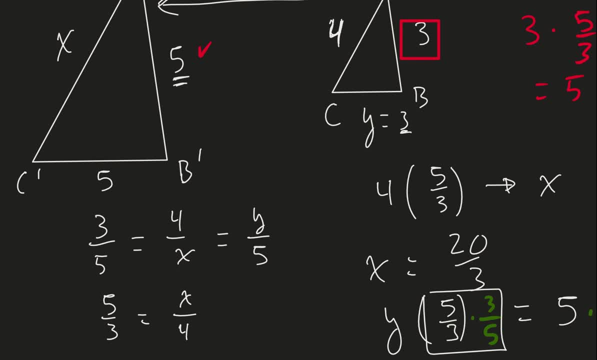 write X over four, and then that equals five over Y. now what's nice about this is that this actually gives me two nice proportions, and I can use those proportions to figure out what x and y are. So here's one of the proportions, And again, a proportion is just a fancy word. 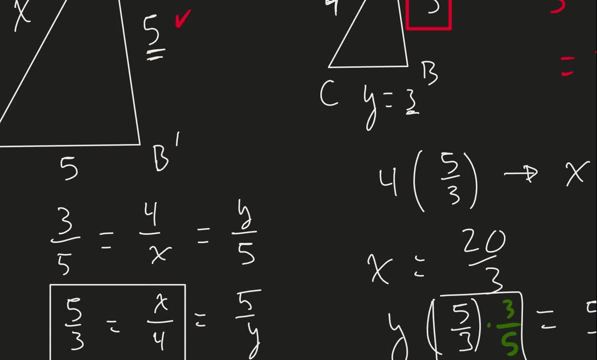 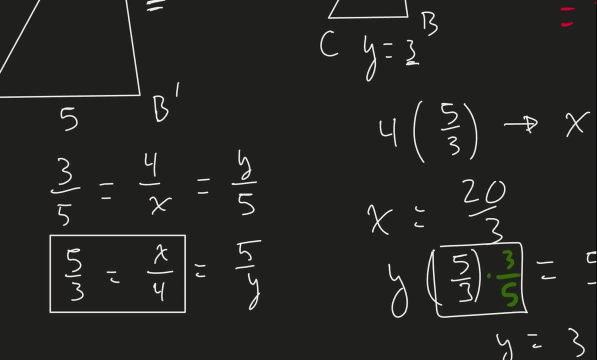 All it means is that you've got one ratio or fraction equal to another fraction. So 5 thirds is equal to x over 4.. When you have ratios like that, we can use fraction busters or we can use the fact that if I multiply both sides by 12,,